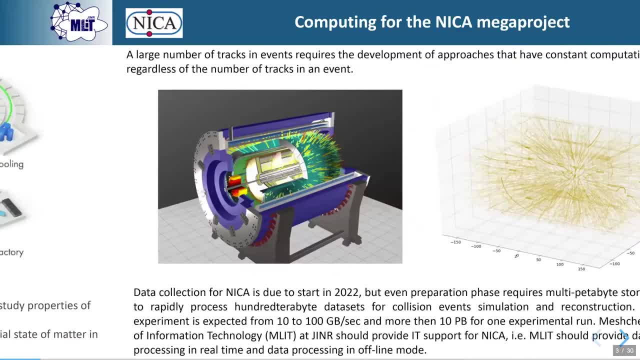 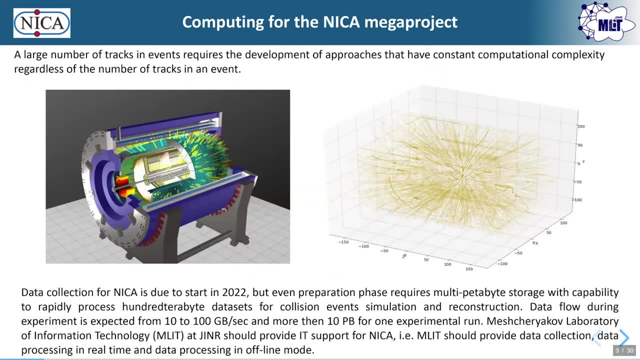 quark-grown plasma and so on. So the event looks like that that we have a detector and in one collision there are many, many particles are produced. We are saving them to the trees or in the future maybe to these aren't apples- And then later on we are just moving them to our trigger system. It is filtering. the event then later on is just post process them. then reconstruction of the events are done by the 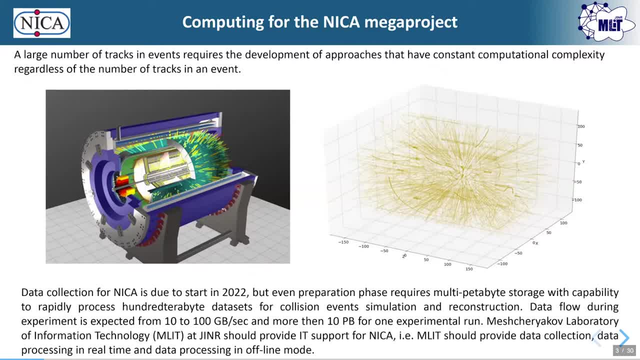 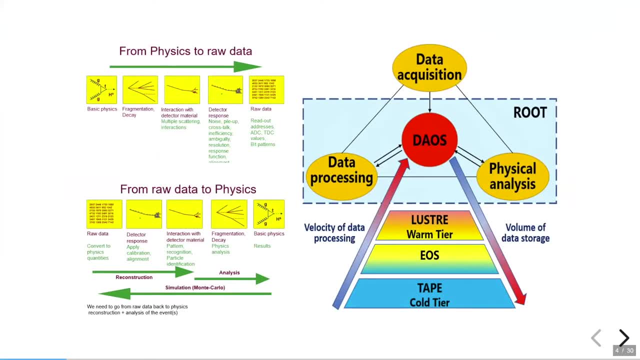 detector and software. there And further on they are doing the calibration And afterwards we might see that there are processes that we are saving the files for the physicists. So just to give you a little bit overview. basically in physics you basically have a model which you have from previous experience. you are trying to simulate on the detector which doesn't exist at all yet, But then you just go and just model it in some 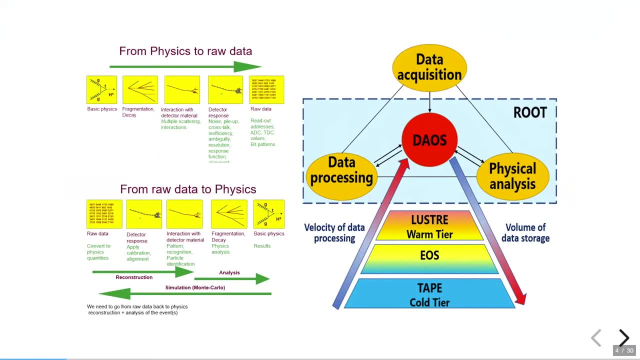 computer. you just process it, do some simulations and at the end you just get some points from the response of the detector. Later on you just process the analysis or you just process the reconstruction, So how it looks like if it would be in the nature and you are coming back to the same histograms and same distributions. Then you compare distributions like it would be in nature and how it would be in the model. then you compare these pictures and 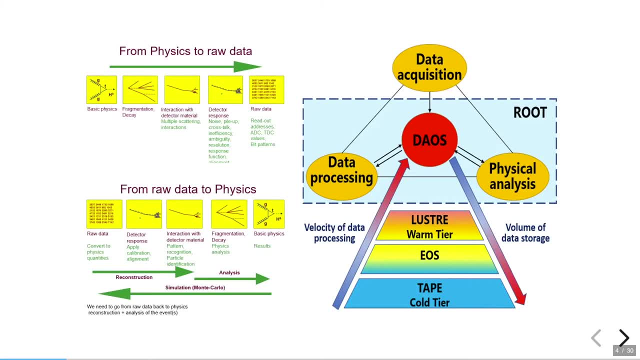 and basically, if they are same, then you might say that your models are working fine. So most of the time what we do, we basically, at the beginning we have a very, very big, high, high throughput from the detector, from the detector to our colder storage. So for that first part we would like to use some very fast storage And, as one can imagine that DDR RAM is very expensive for that, So we would like to use DAOs for that, just to do that. 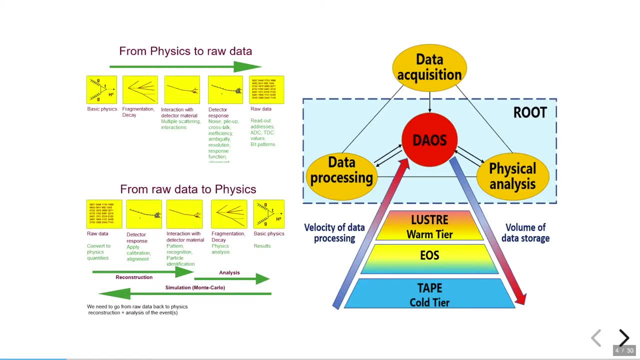 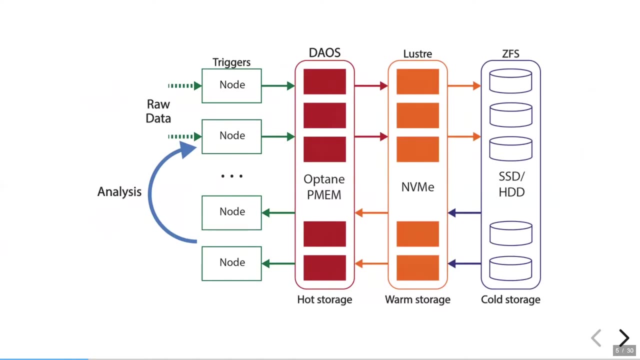 And later on what we do. we simply we have the first term that we go from the raw data via trigger to DAOs and then to luster When the data is ready for the physicists. they are going to and read this from this colder storage. They are just reading it, then process it on the huge cluster. 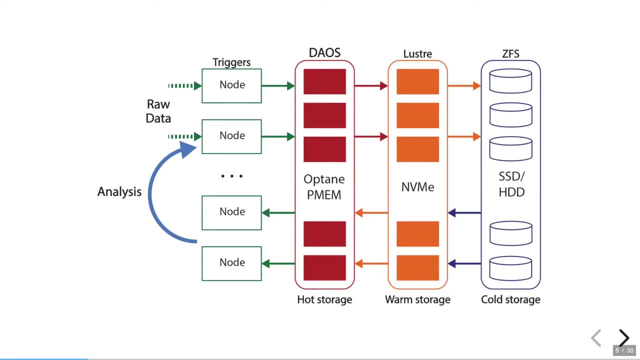 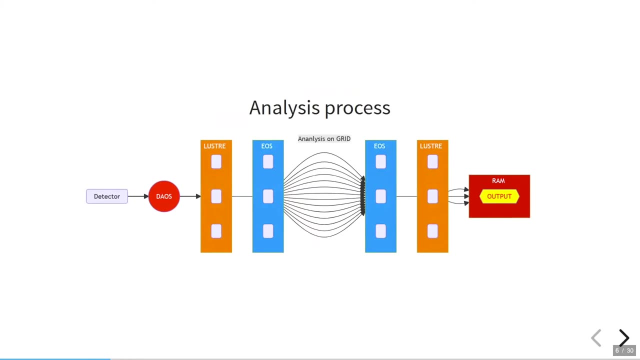 read and then later on they are also stored back to the colder storage and then post-process them on their laptops. So let me do this two-way turn and introduce you into that picture. So at the beginning you have this detector, DAOs, elastor, storage. So let's assume that physicists 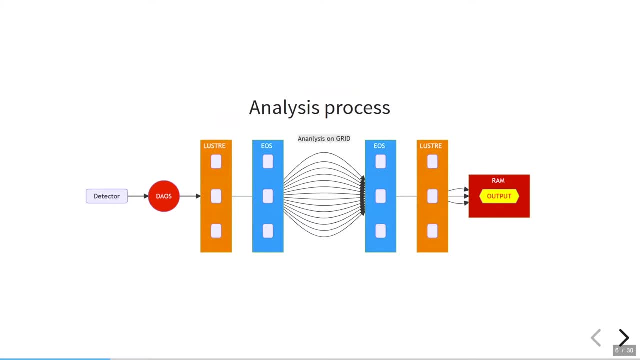 are going to process their data. So what they do? basically they are reading from ELs or elastor storage storages, which are distributed all around the world in the computing trunk which is called GRIT. So basically what you can see here that we are just submitting. 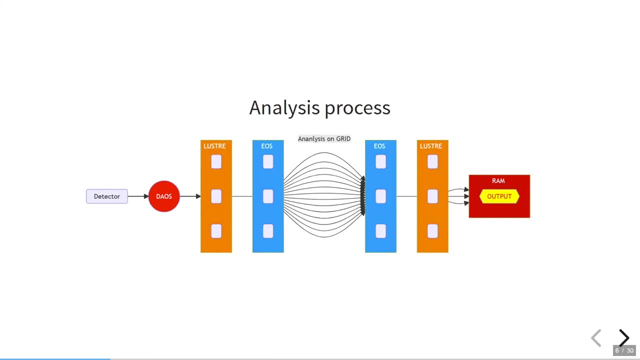 many, many jobs, since events which are we are analyzing are independent from each other. We can do it and we can scale perfectly. So we just submit many, many jobs. we just process these events, which takes basically hours or sometimes days to process the data. 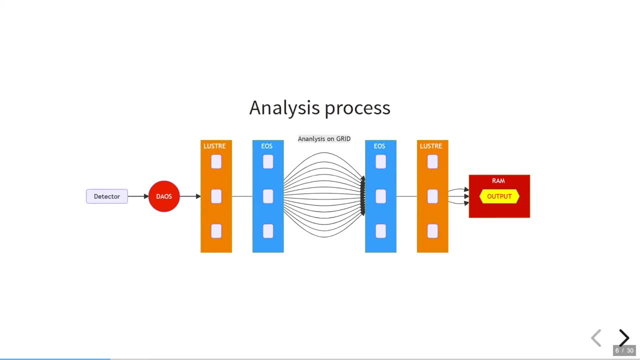 So let's take a look at the data that we have here, post, process them and later on we copy these results, sub results, to the colder storage, and next step, we are just uh, merging these results like it is shown at the end and basically the the physicists at the end, they just open the final objects in form of histograms. they open them in. 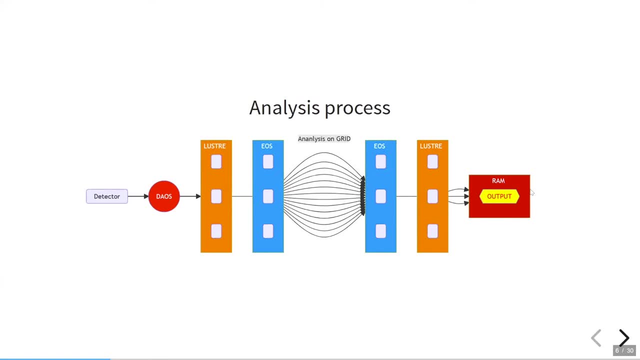 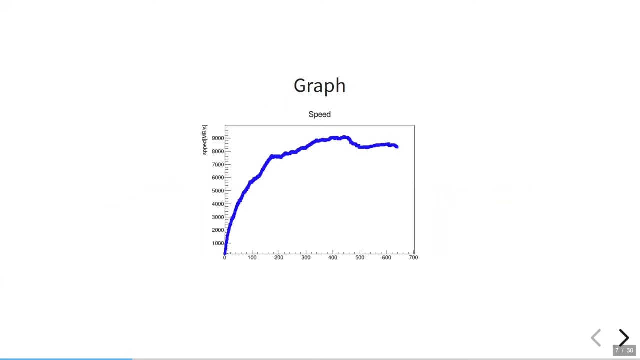 their laptops, basically, and then, uh, just producing the pictures for publications. uh, so just let me explain what histogram means, what we have in mind, that, for example, let's assume that we have some, some graph like that that you have on the x-axis you have a time, and then on y-axis you have some. 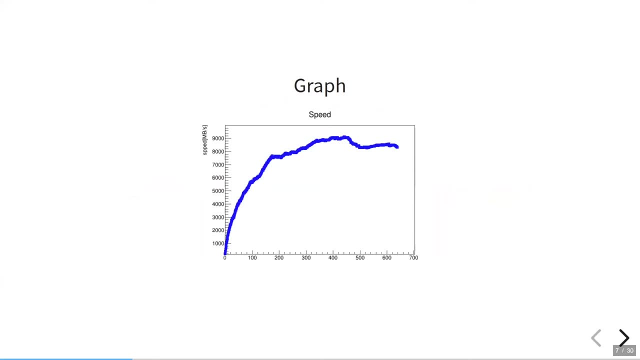 parameter like speed. so this is what you can be like. this is the how it goes. this is very. i was measuring the dallas system tests and this is my distribution of the speed. so what we do, basically you have that one and then to create a histogram out of that, because sometimes you are not. 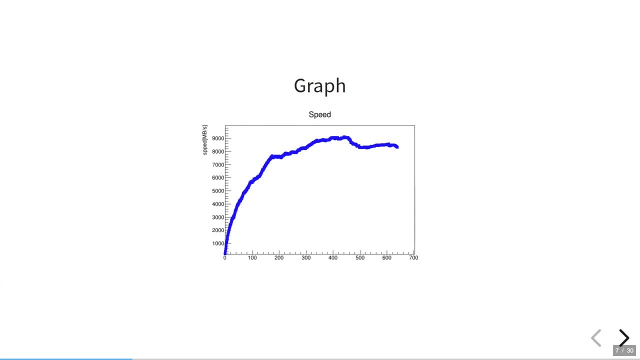 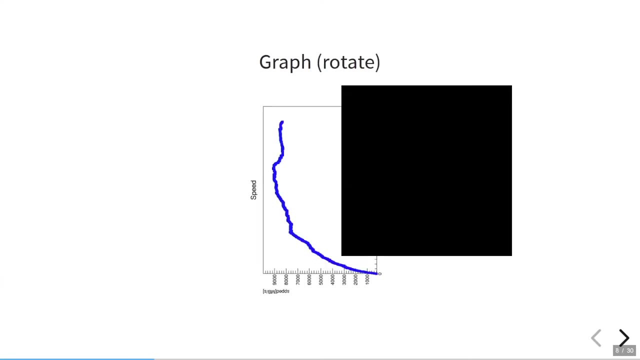 interested in time because you are not interested in time. because you are not interested in time like to find out that how often you were at the highest speed, or whatever how the speed is distributed. so what you can do is simply rotate the picture once second. you then mirror it and 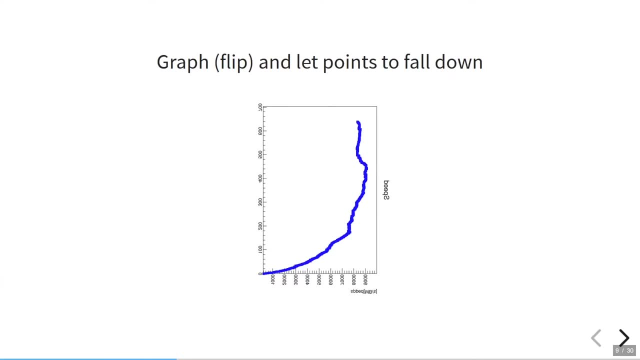 then you just let all points fall down, uh to the bin, uh axis and then you have something, some distribution, something like that. so this is what you can see. this is the same picture, but we can see that mean value for the speed is seven point uh, four gigabytes per second. this is how we. 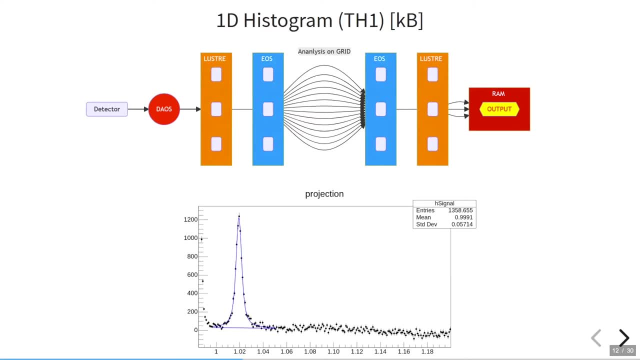 use histograms. so in our picture it is like that. so we simply do, uh, do the same process. so, as you can see, the same thin line are shown in the great analysis. so that means that object is small. basically, when people are physicists, are running the process, then they are just if they are, if their. 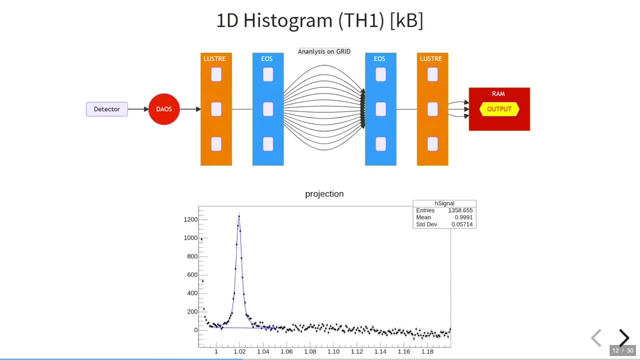 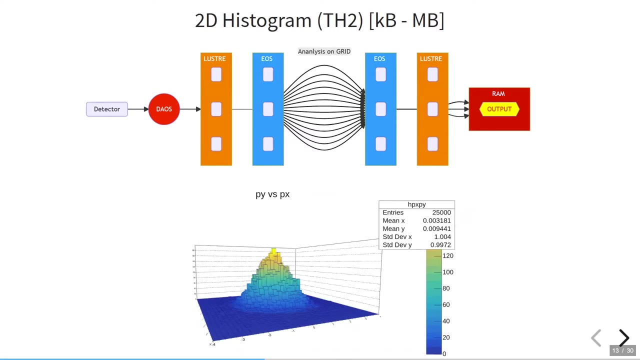 output is in form of one d histograms. basically they are kibble bytes, so there is no problem to merge them and and process them at the end in the in their laptop and just show the results. uh, but since the, the analysis on the grid takes hours and people would like to analyze the multiple parameters at once, so what they do. 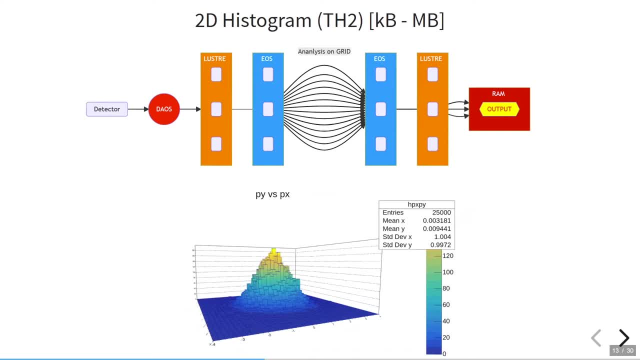 they are just increasing dimensionality in the histogram: uh to get to, to run, process uh in the grid only once and then just save as much information as is as it is possible. but this is what is happening for two-dimensional histograms. but when you go more and you are 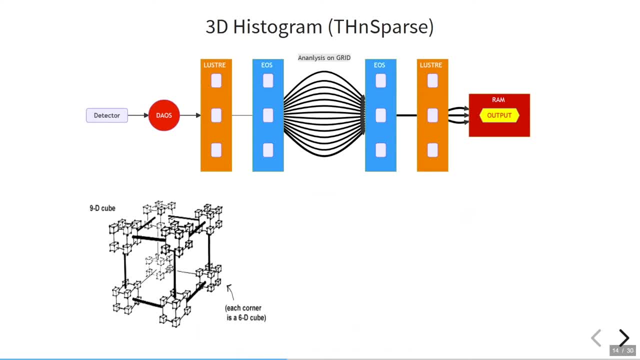 doing more and more axis, so more it consumes in the memory of the computer at the end. so this is how you can do, then, what you have to start to think that you don't have. you cannot reserve a memory for whole histograms, because if you have three-dimensional, for example, you 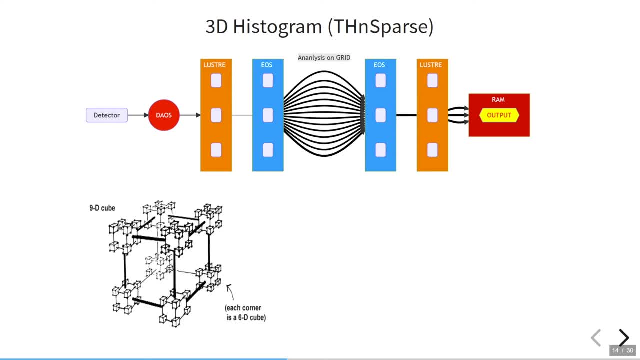 have thousand bins times thousand bins and times thousand bits. that means like eight bytes for double. so that means that you have already eight gigabytes of memory. so that's why either you store it in the laptop or i mean, you have to open it. you have to be able to open it. so for that we're. 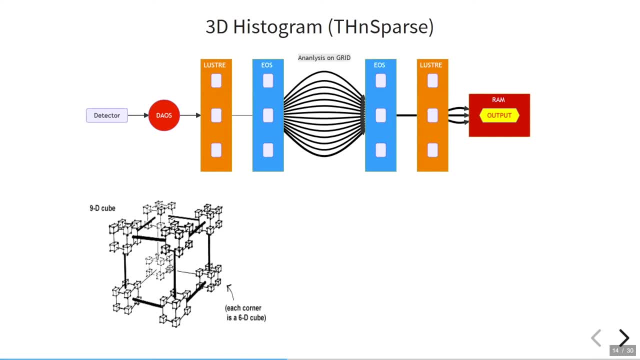 we are, and root has the possibility to do th and sparse objects, which is not reserving memory at all, but only when the bin is filled or some information is there. but in that case you have a nice job that you can simply have very big histograms, not fill them fully in the grid and 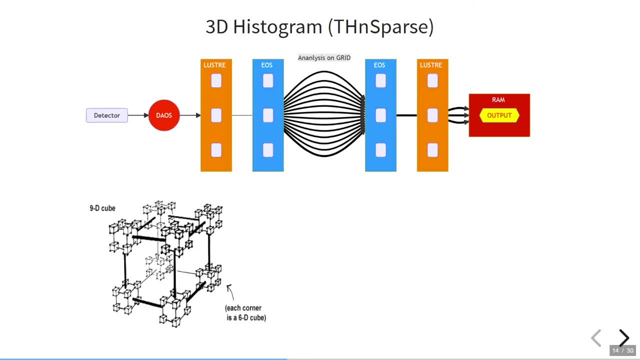 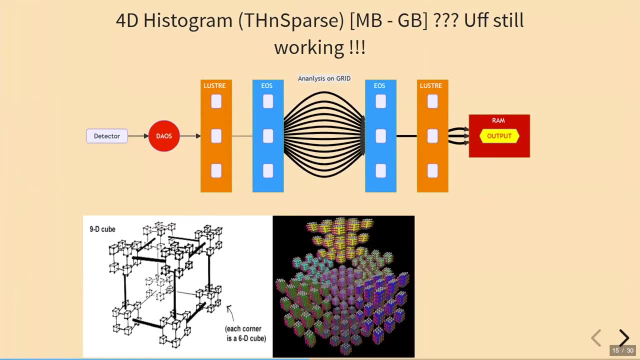 but at the end you might reach to the point that the objects at the end might be much more bigger than it is on the single job in the grid. so what happens then? you have, whenever you are increasing number of axis, that means that you are wearing that you are not going to fit in memory. so what? 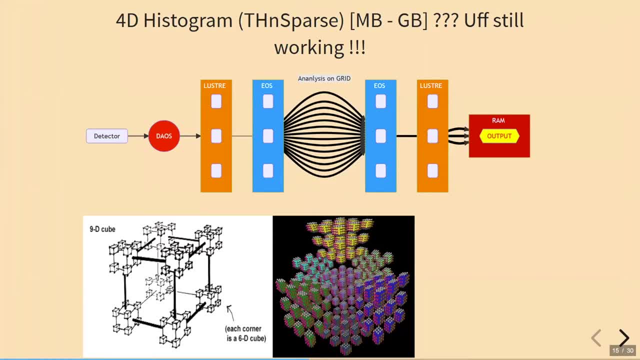 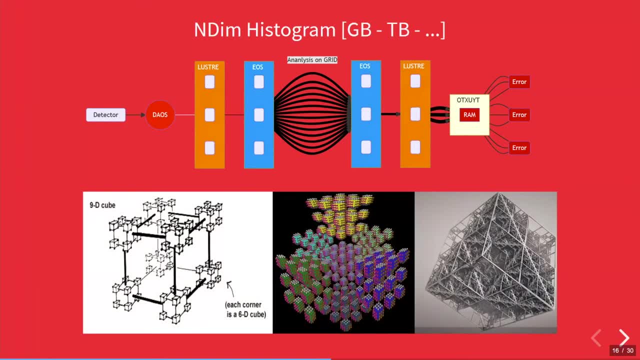 they what you do. basically, you just lower the resolution of the histogram or something. but what you would like to do, we would like to go more, deeper and deeper. anyway, you will hit the point. so that's why if you are increasing the size of the uh of the histograms, then your output is wrong. 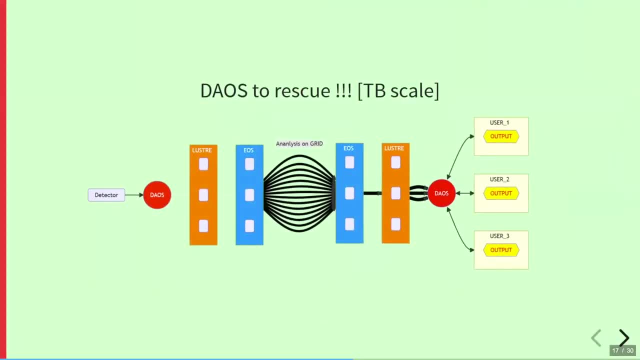 or you are not able to open it at all. so for that there is a douse which is here to rescue us when histogram is in terabyte scale. so what we can do, we can just store it and to the, for example, key value storage, and then we can just have it there and then later on, multiple user access can access. 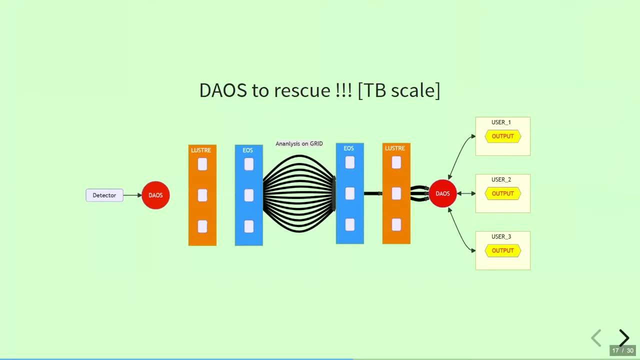 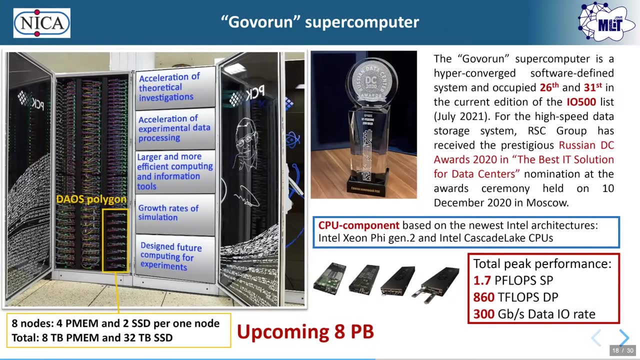 and do the projections of different physics. so we have the, the super computer gavaron, in our computing center in dubna and where we have the douse which is taken, uh, eight nodes and 32 terabytes, and the next eight petabytes are coming. so this is what our tests, we were doing on that one. 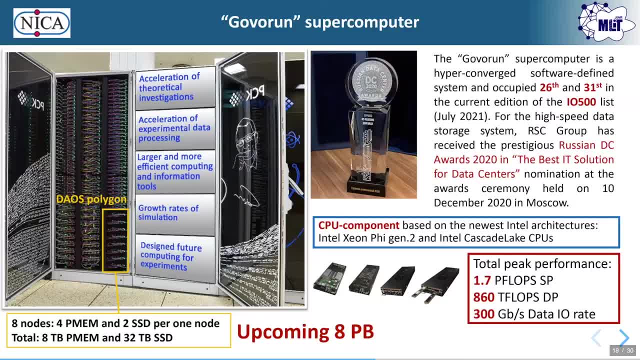 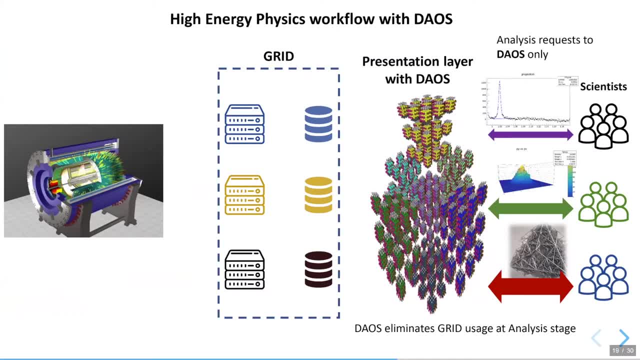 because what you have to do, first you have to check the implementation, and so this, this kind of things. so what i would like to mention here that, uh, at the beginning we are, we have this processing on the grid, but later on we have this presentation layer which dallas can store for us. 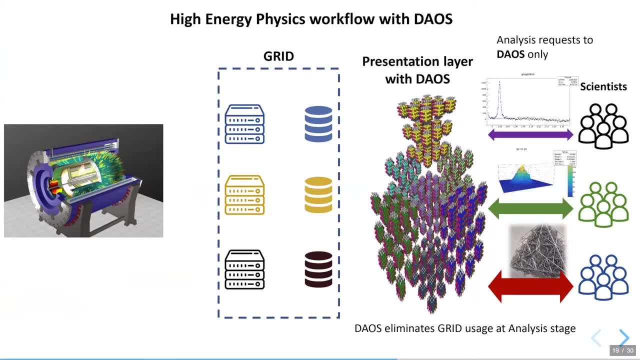 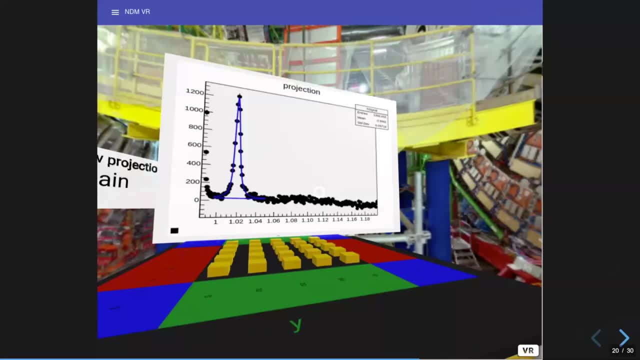 and later on it can be used from the physicists. so this is very important part which we are working on in our project, which is perfect, is perfectly fitting to our process workflow. so when, at the end, one can see the in virtual reality, we have the ndr project which we are. 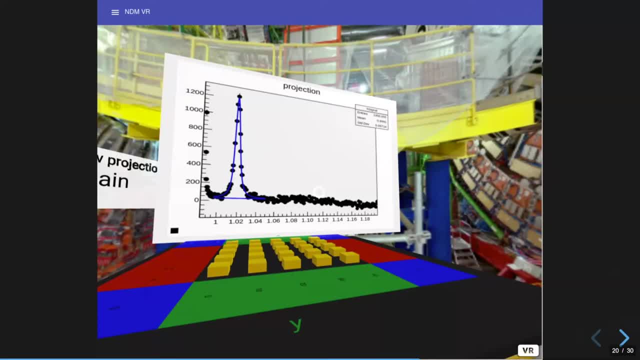 working on that, that physicists can simply go and click on the some bins and the projections are done that way that simply when someone will click on the bin, then it is calculated on the cluster, then the query dows file system. uh, to get the projections, then do some fittings and return. 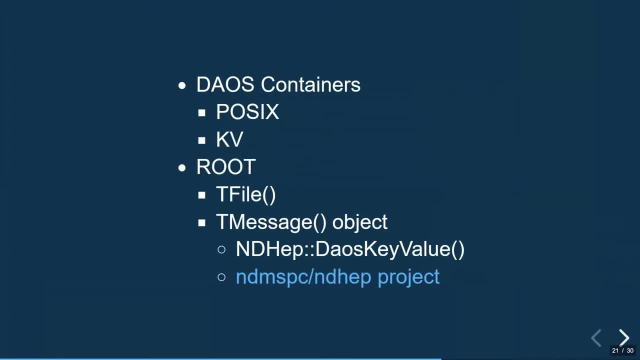 points. uh, at the end i will show you the demo. um. so in our cluster we we tested two type of containers: uh, bosex and key value. so bosex is very similar to eos, which we are having the at cern or in dubna, and we have the root object, which is called t file, which is basically the file objects. 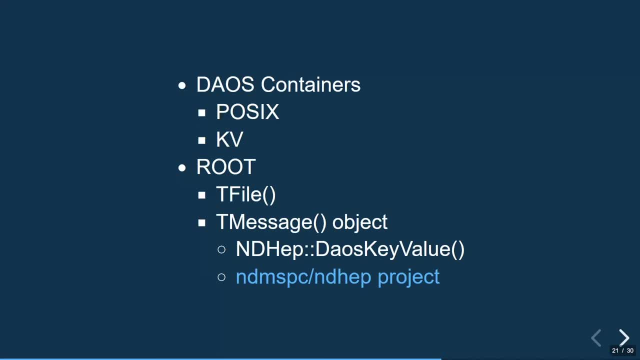 which is stored there. so for posix, we use t file object to store these uh big histograms there, and i also. we also implemented the dallas key value object, which is basically using the message object where users can save any root objects to the bytes and then 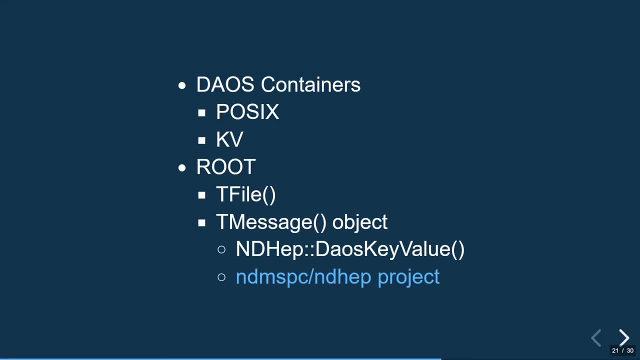 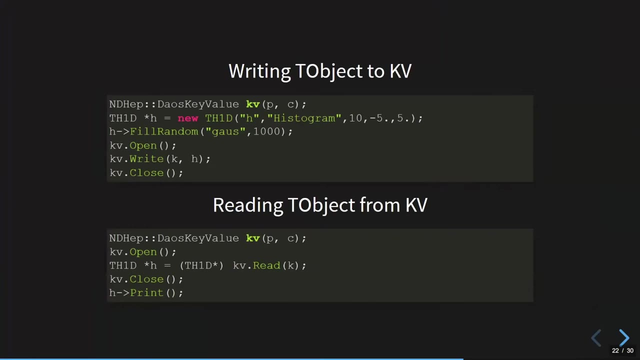 we convert it to the via DAOs API interface via bytes to restore it into the p-value. So implementation is there in this and we have projects. one can look at each one. So the ideas are that simply, you just create a p-value object. 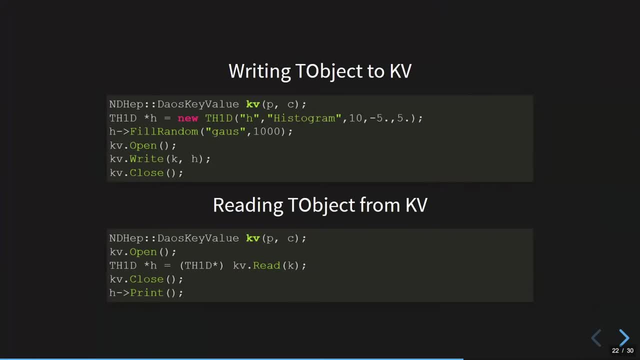 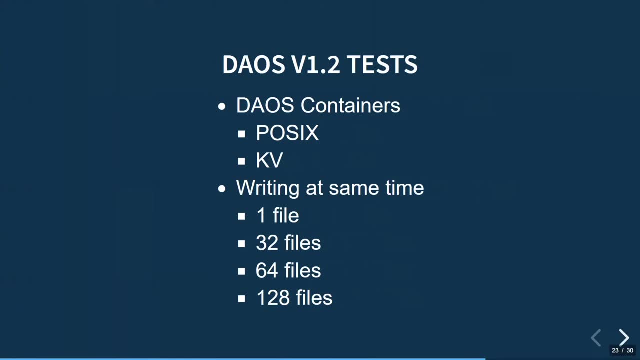 you create some histograms, open it, then write it and close it For reading. it is very similar. you just use the read function. So we were using DAOs 1.2 and what I was doing, that- I was testing that at the same time from these: 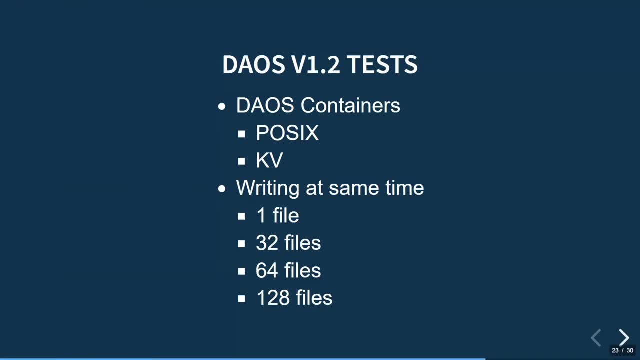 eight nodes. we basically were writing one file, 32 files, 64 files and 128 files at the same time. So just for the test to be bigger, that on one node I was writing multiple files, but I mean at the same time you're writing that many files. 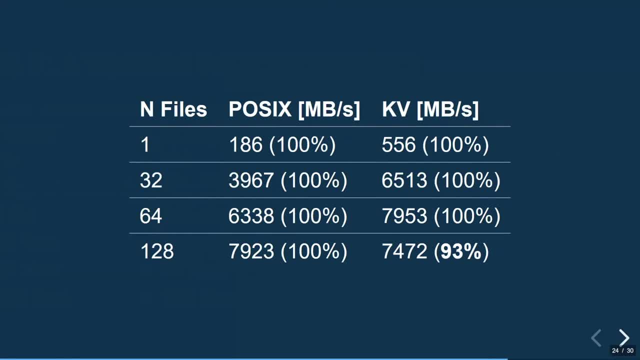 And these are the results. so, as you can see, the POSIX is a little bit slower when only one file at the same time was written. This 100% means that 100% of files were written correctly. So whenever we wrote 32 files at the same time, 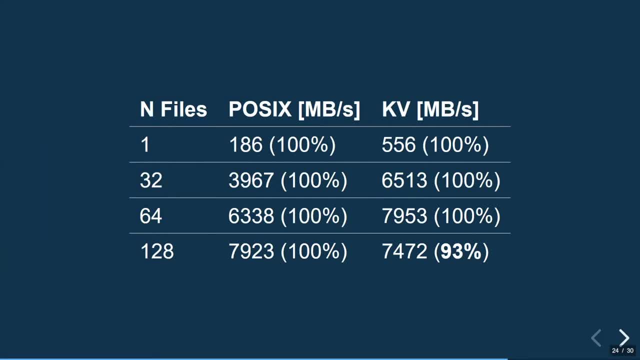 so almost 4 gigabytes per second for POSIX and p-value has the 6.5 gigabytes per second. So for 128 we were reaching a almost eight gigabytes per second. but for key values we were also reaching the speed almost, but we were starting to have some failures in when that key key or the object to the current key. 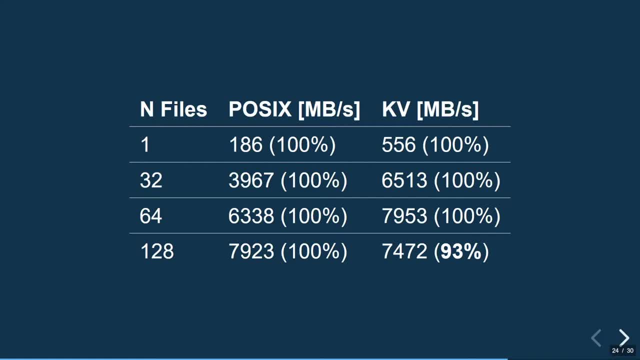 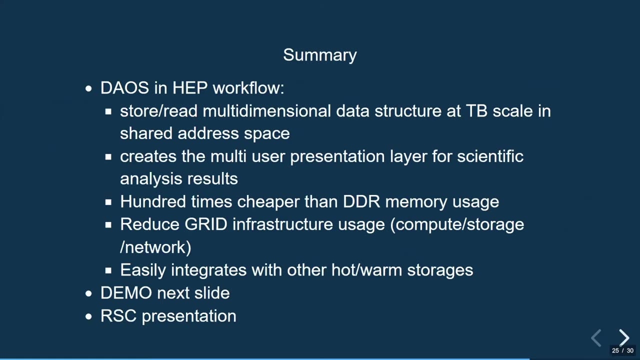 was not stored, but i think maybe it is because of the version or some bugs there, or maybe there is some configuration in our network. but okay, let's, we can improve that later on. so i would like to summarize that that in high energy physical workflow we can store and read multi-dimensional. 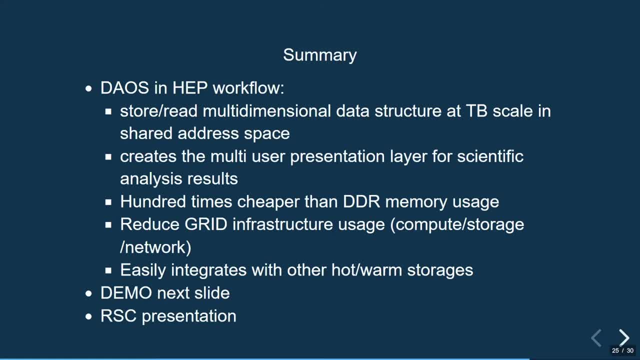 data structure in terabyte scale in shared address space to create multi-user presentation layer for scientific analysis results and it is 100 times cheaper than ddr and it will reduce the in grid infrastructure usage and also it will interact integrate with the colder storage. so here i would like to show you some demo with with this 3d view and then later on anton can have a. 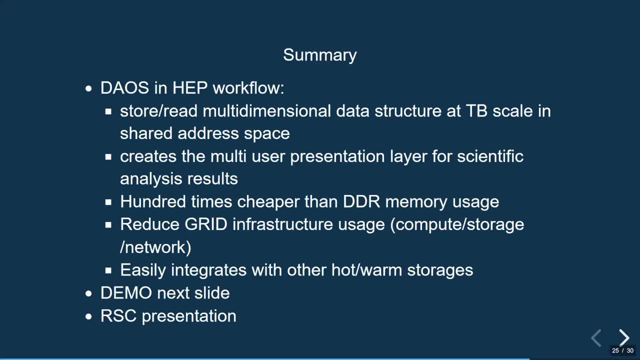 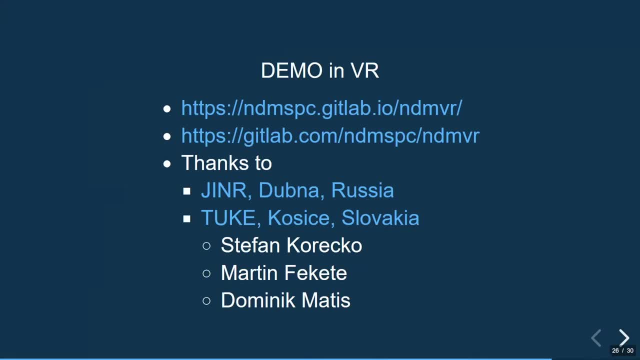 presentation. we are implementing the project in the gitlab, and so one one- look at the first link- you can basically do the same thing what i am doing now, and then there is a source, and i would like to thank a technical university in kosice for students who were doing the implementation. 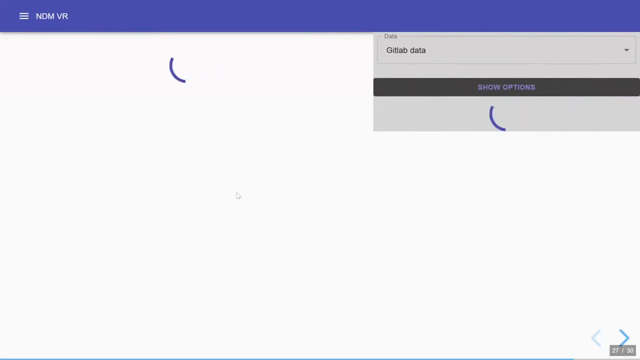 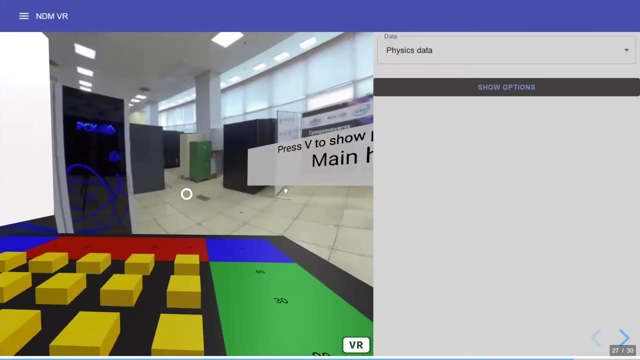 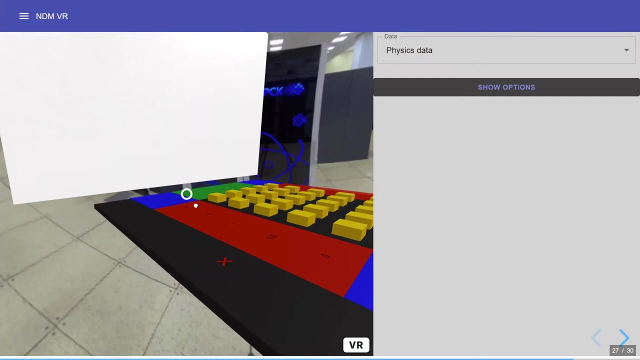 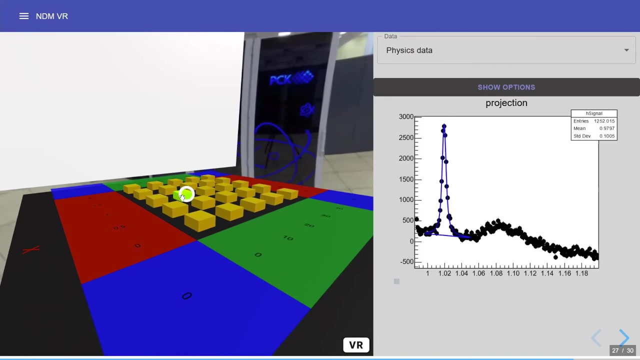 so let me load the interface. so here i would like to show you the the physics data, so you can, you can move there like you are in minecraft. so basically the commands are uh useful, like for moving. then later on when you click, click on the pin. oops, okay, sorry, so once more, all right, let me put light in my side, okay, so, so when you click, 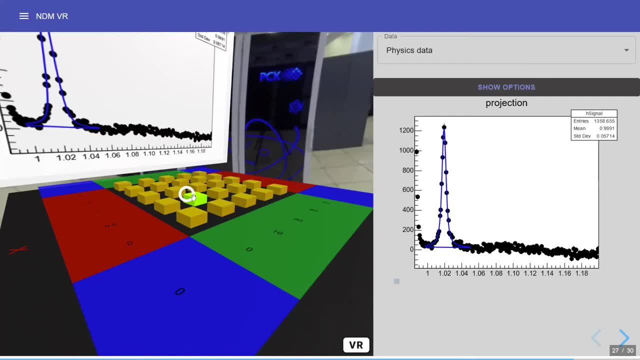 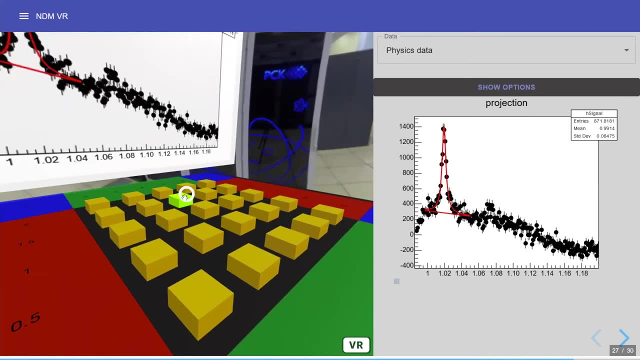 you can see the projection over the bin. then process uh is fitted and physicists can look over different bins. for example, in our case, whenever the color of the fitting function is red, then it means that fitting somehow it's wrong and physicists can basically with some simple button find out what fits are okay or not. they can adjust it and 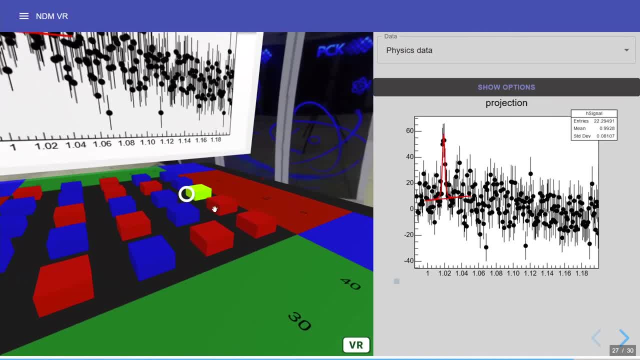 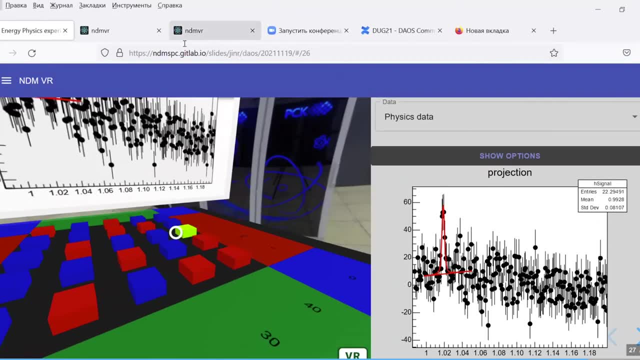 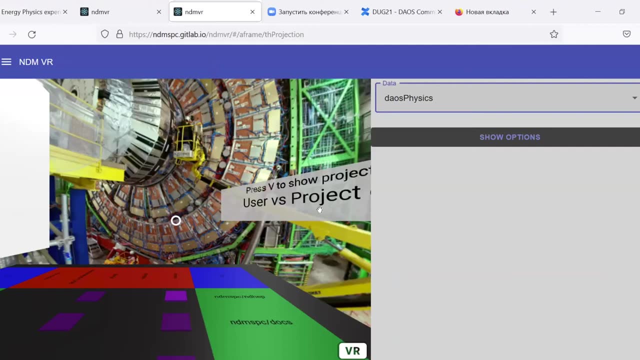 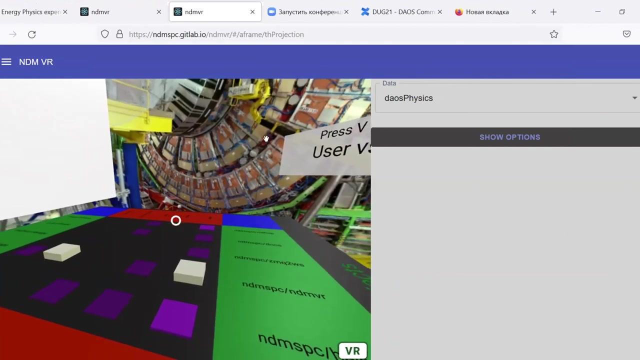 simply run it again. so, as a as a second demo, i would like to show you sorry, okay, like this: yes, i think you get the point and i will leave the presentation for anton and then later on maybe, if you have a question, i can show you more stuff. so thank you very much. 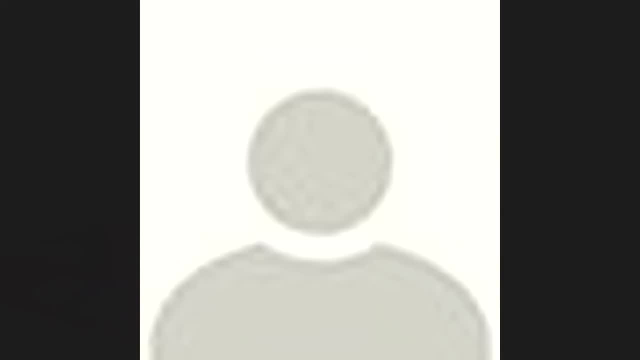 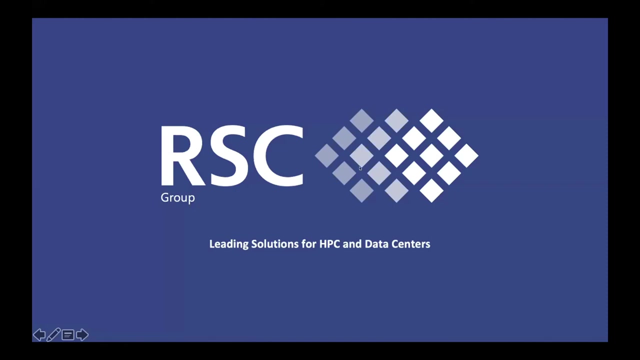 anton, you can take this. yeah, can you. can you hear me? yes, yes, okay, um, just a second. uh, are you seeing this? yeah, i can see the slide. yeah, i will be quickly. um well, uh, thank you, martin. um, hello everyone. my name is uh anton. i'm working for rsc group. uh, at first. 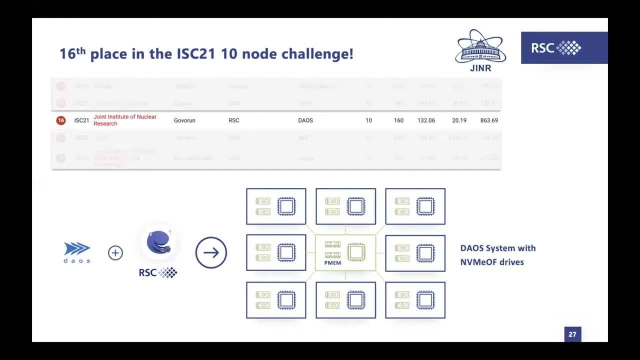 at the web item families website, um, and in this video이에요ove stock frusti. it would be great to. i want to remind that on the previous dog we talked about dallas in the context of our orchestration system called storage on demand, and we said that it would be great to use, and we mean of. 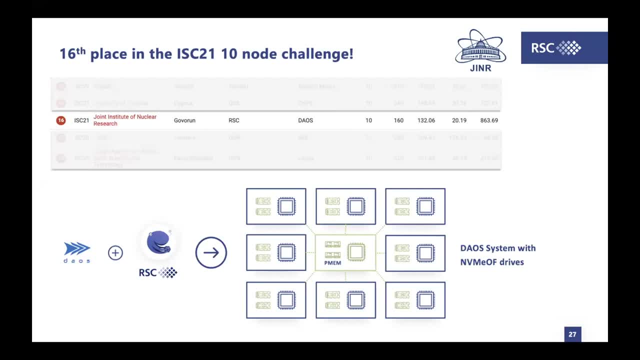 fabric drives instead of directly attached en vimi drives, and first of all, it helps to remove um the hardware limitations and also helps to create more flexible configuration of- i turn my magic away close-up here, if not it is mustache- drawing my colleagues from Jenner and RSC. 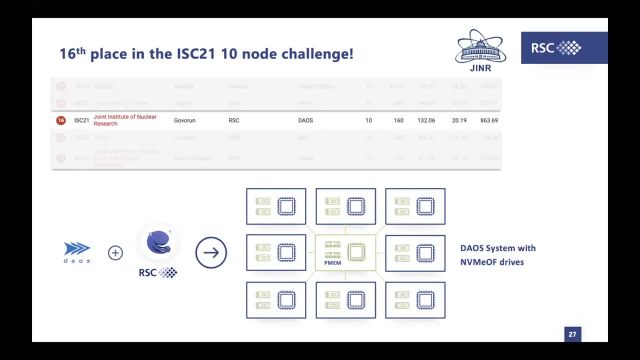 built a DAOS with the NVMe fabric drives using our orchestration system and we took the 16th place in the ISE 2110 note challenge. I want to say the big thank you for the DAOS team, for the DAOS. 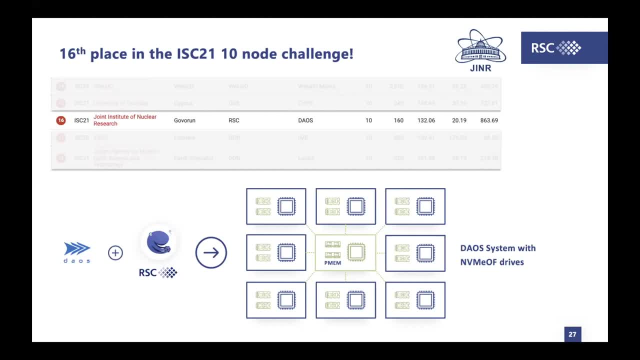 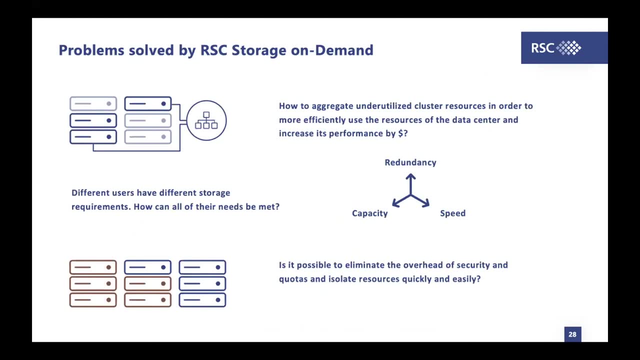 community. They helped us a lot with the debug. So the problems we solved with our product: first of all, it helps to pull underutilized cluster resources and use them more efficiently. Second, it helps to meet the needs of the different users with the different 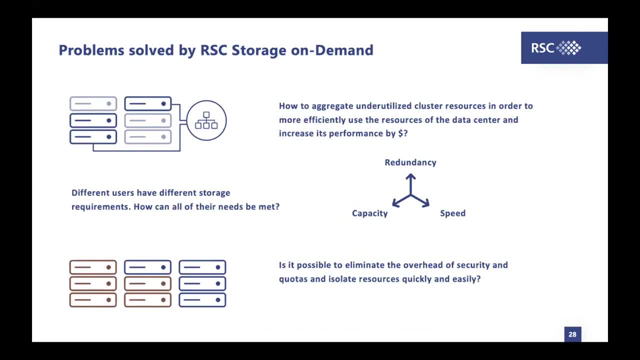 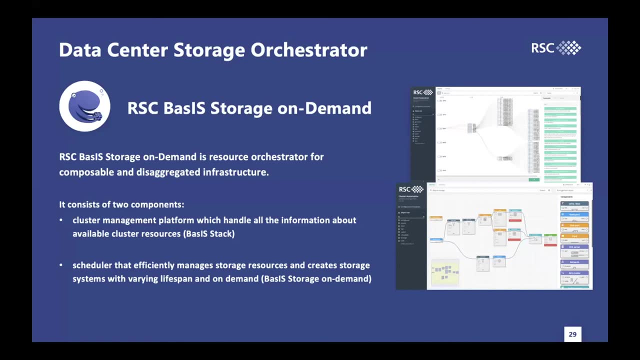 storage requirements. And the third and the last, it allows to quickly and easily isolate resources, while we create storage for a specific job or person. Well, our system consists of two parts. The first one is the cluster management platform that stores all information about the available cluster resources. 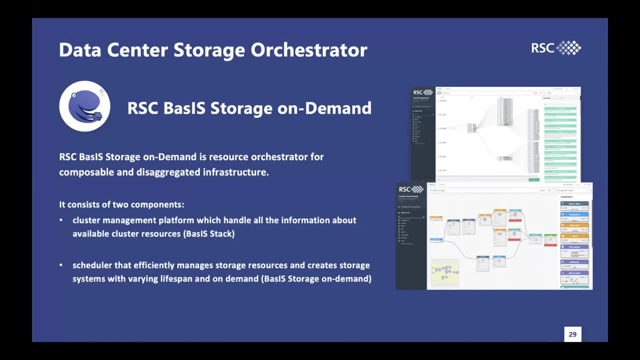 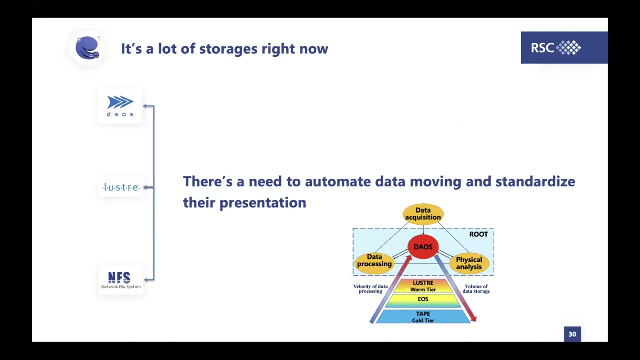 called the BASIS stack, and the storage on demand part, which is flexible scheduler that manages the storage resources and creates storage systems on user demand. And the last slide, as Martin mentioned. now we have already a lot of storage. We have a lot of storage.